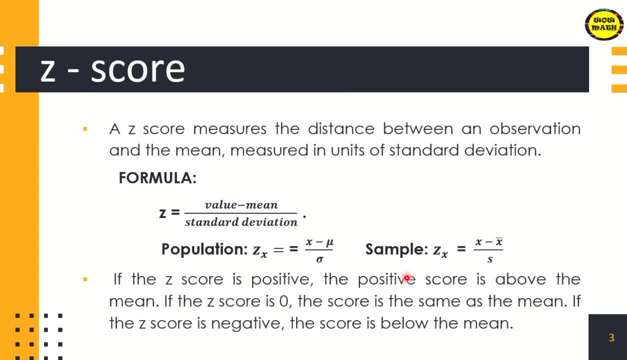 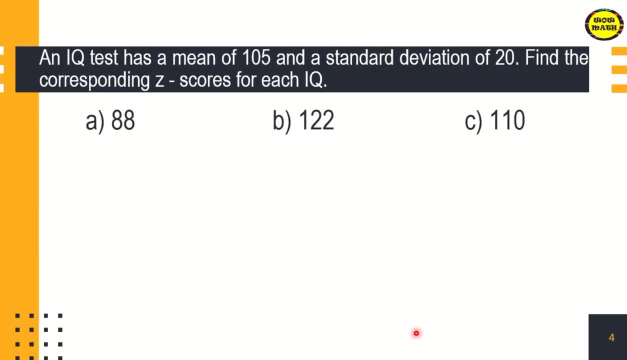 Again, If the z-score is positive, okay, meaning that the score is above the mean. If z-score is zero, the score is the same as the mean, And if the z-score is negative, the score is below the mean. For example, an IQ test has a mean of 105 and a standard deviation of 20.. 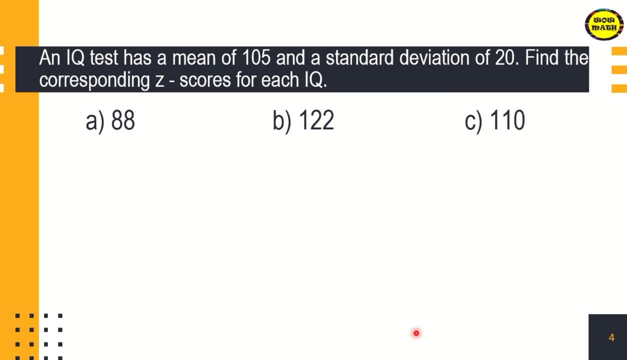 Find the corresponding z-scores for each IQ. So first the score is 88.. So using the formula value minus the mean over standard deviation. So let's just substitute. So that is 88 minus 105.. So the value of mean is 105 over 20.. 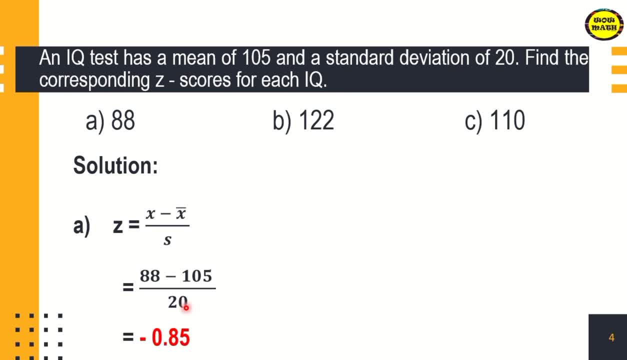 Or 88 minus 105 divided by 20.. So the answer is negative, 0.85.. Since the value of our z-score is negative. so therefore 88 is Below the mean, Next 122.. Okay, If our score is 122, same process. 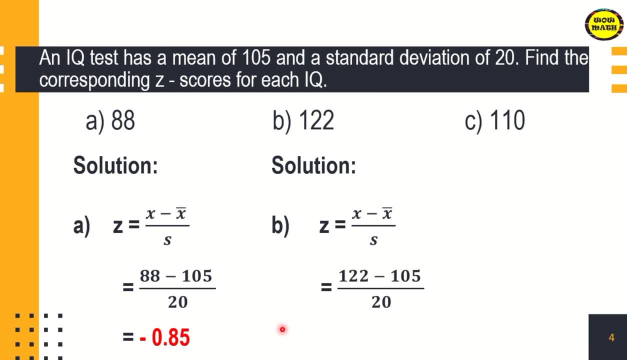 Using the formula, we substitute 122 minus 105 divided by 20.. So 122 minus 105 divided by 20.. The answer is 0.85.. And 0.85 is positive. Therefore, 122 is above the mean. 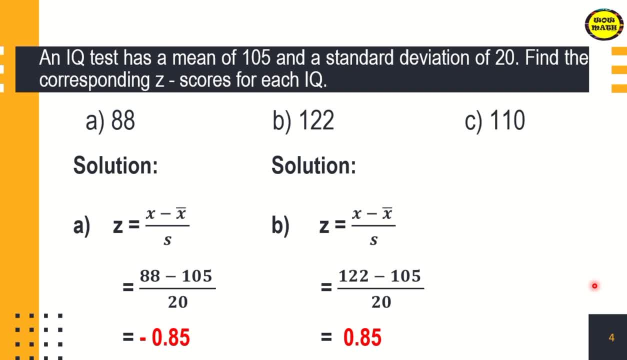 Next 110.. Same process, Using the formula, we're going to substitute 110 to our x, So that is 110 minus 105 divided by 20.. So 110 minus 105 divided by 20.. That is 0.25.. 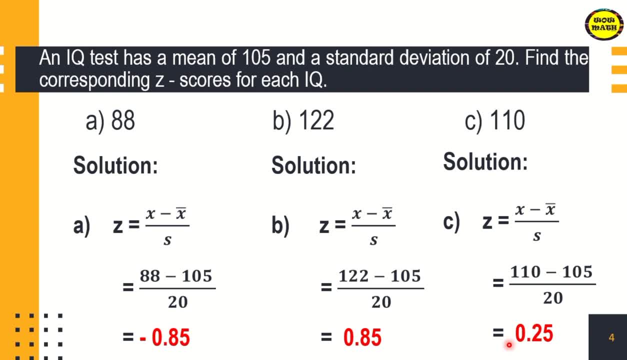 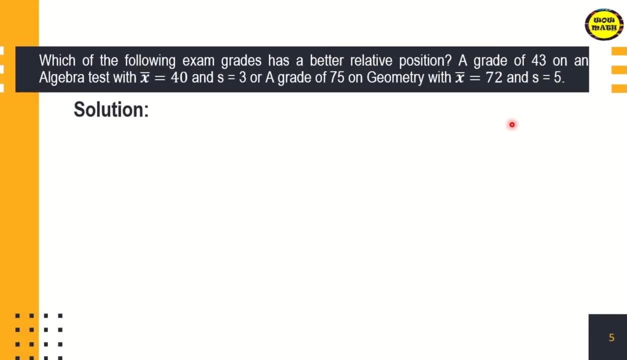 And then 0.25 is a positive number, So meaning our z-score is positive. Therefore, 110 is above the mean. Next, Which of the following exam grades has a better relative position: A grade of 43 on an algebra test with a mean of 40 and the standard deviation of 3?? 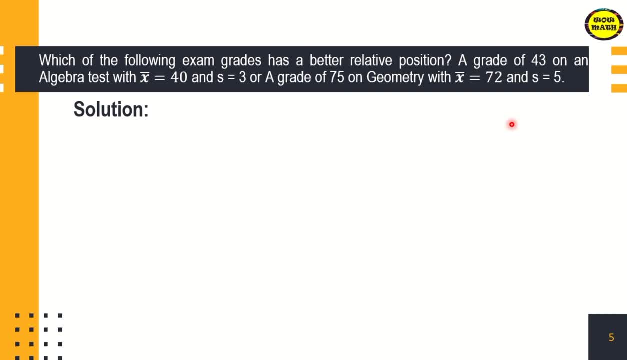 Or a grade of 75 on geometry with a mean of 72 and standard deviation of 5?? So in order to find which, Which of the following exam grade has a better relative position, we need to find out the z-score of the two tests. 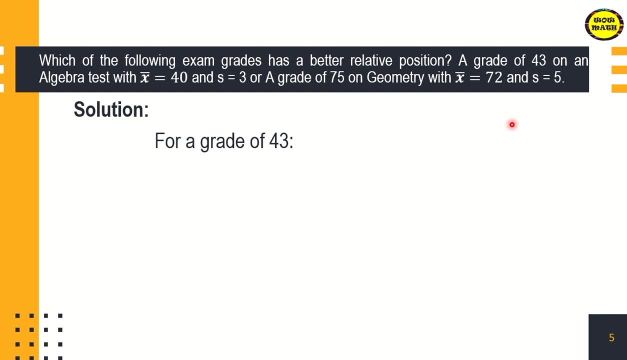 Okay, First the algebra test with a grade of 43.. Okay, Let's find out the value of the z-score. So 43 minus 40.. Why 40?? So that is the mean value. So 43 minus 40 divided by 3.. The answer is 1.. So in algebra 40 is the mean value So 43 minus 40 divided by 3.. The answer is 1.. So in algebra 40 is the mean value So 43 minus 40 divided by 3.. The answer is 1.. 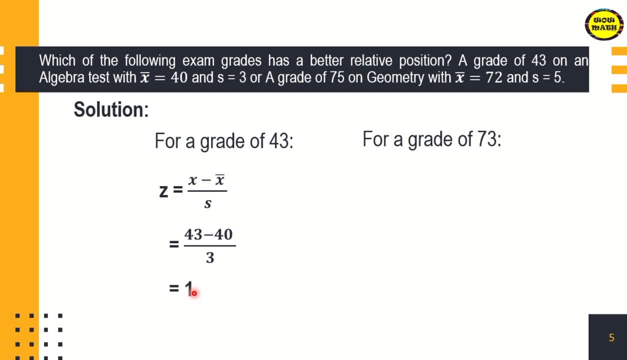 In algebra test, the z-score is 1.. Next For geometry test, with a score With a grade of 73.. So that is what. After that, a grade of This is Okay For a grade of 75, for geometry test. 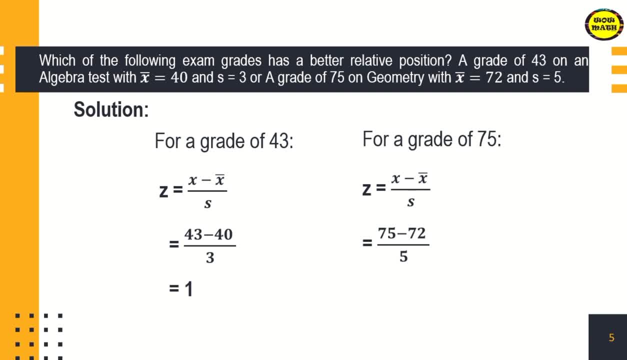 so that is 75 minus 72 divided by 5, and that is 0.6.. Okay, So what do you think? So which of the following exam grades has a better relative position, Since in your algebra test the z-score is 1,? 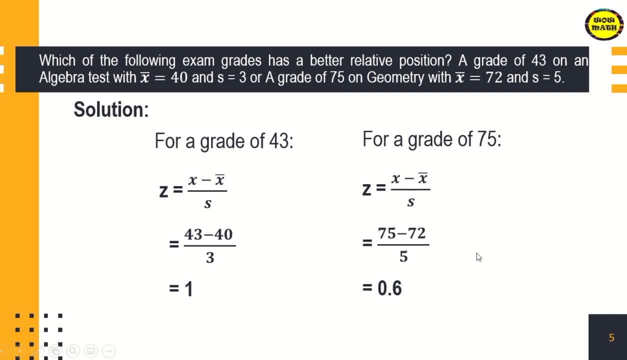 and for geometry grade no, that is algebra yeah, And for geometry that is 0.6.. What do you think Okay, since the z-score for the algebra test is larger. the position in the algebra test is higher than the position in the geometry test. 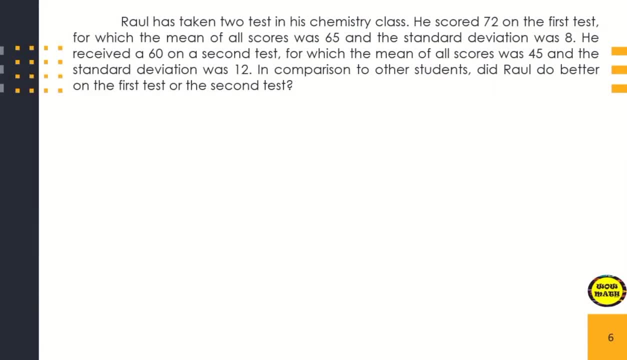 Okay, another application. Raul has taken two tests in his chemistry class. He scored 72 on the first test, for which the mean of all score was 65, and the standard deviation was 8.. He received a 60 on the second test. 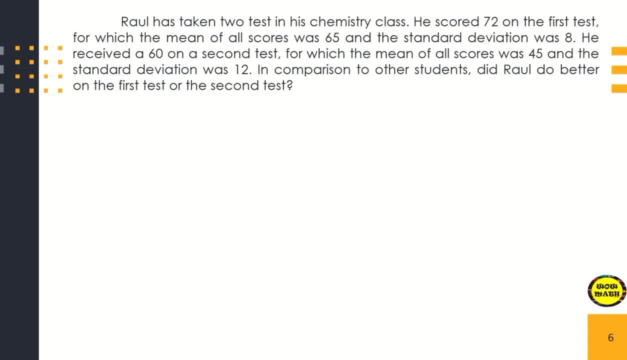 for which the mean of all score, the z-score, was 45, and the standard deviation was 12.. In comparison to other students, did Raul do better on the first test or the second test? Okay, let's find out. So for a score of 72,. 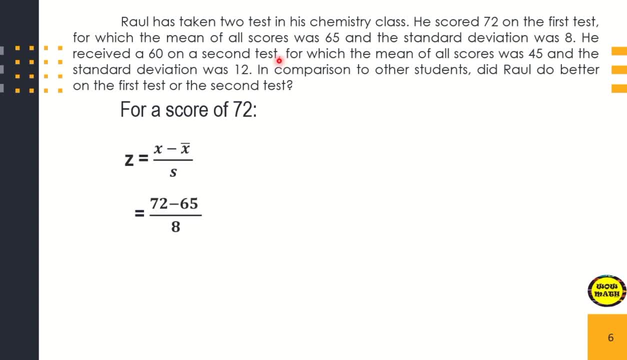 so 72 minus 65,, since that is the mean of all score, so 65, and the standard deviation is 8.. So 72 minus 65,, that is 0.875.. Again, 72 minus 65 over 8,. 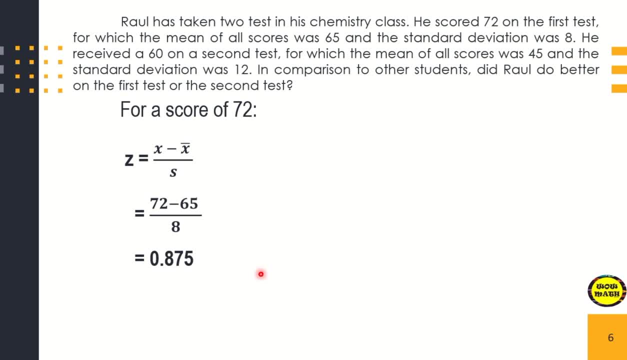 that is equal to 0.875, and that is for the first test. Next is for the second test, with a score of 60. So that is 60 minus 45,, since the score of Raul on the second test is 60,. 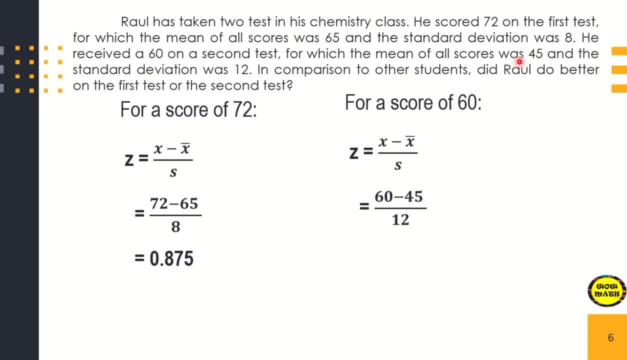 minus 45,. that is the mean of all score in the second test. 60 minus 45, divided by 12.. So that is 1.25.. So therefore, did Raul do better on the first test or on the second test? 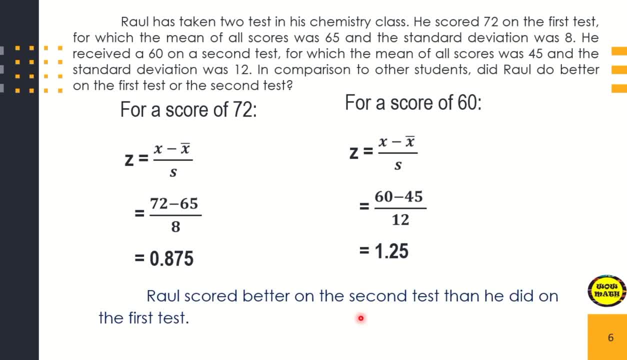 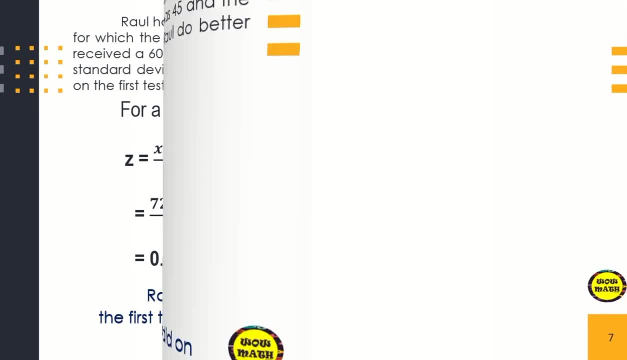 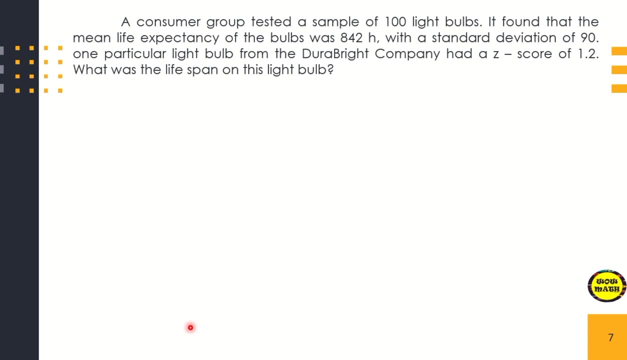 Yes, Raul scored better on the second test than he did on the first test. Okay, another class. what if the z-score is given again on the problem? okay, Like for example, in this problem, a consumer group tested a sample of 100 light bulbs. 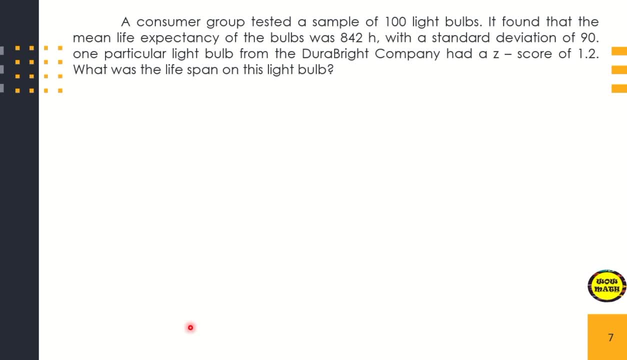 It found that the mean life expectancy of the bulbs was 842 hours, with a standard deviation of 90.. One particular light bulb from the DoraBrite company had a z-score of 1.2.. What was the lifespan on this light bulb? 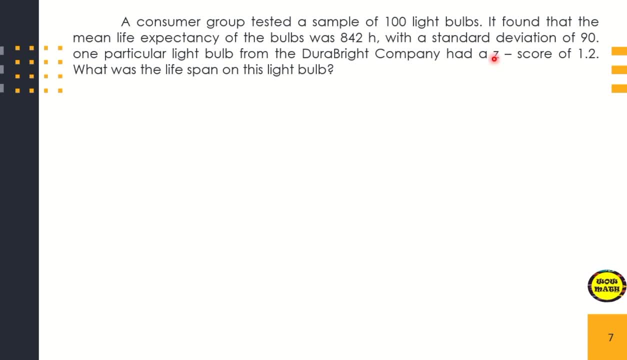 Again in this problem. okay, the value of z-score is given and that is 1.2.. So how we're going to so meaning x is unknown in this problem. So how we're going to do it. 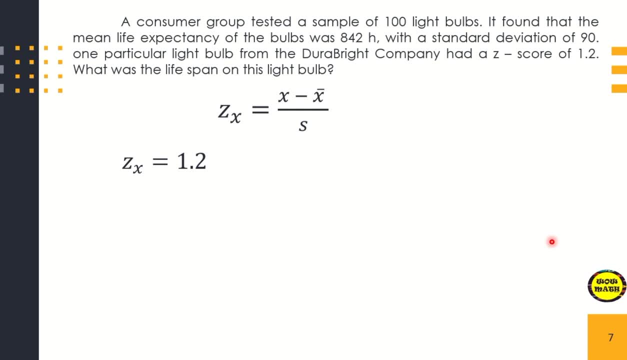 Applying same formula. So let's get first the given value in order to find the value of x. So the z-score is 1.2, and the value of the mean life expectancy of the bulb was 842, and the standard deviation is 90.. 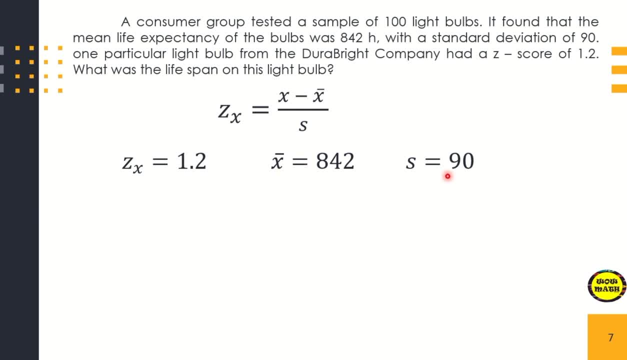 So, using this, the three givens, so we're going to substitute in the formula. So 1.2 is equal to x minus 842 divided by 90.. So if this is the equation, we are going to apply the LCD. 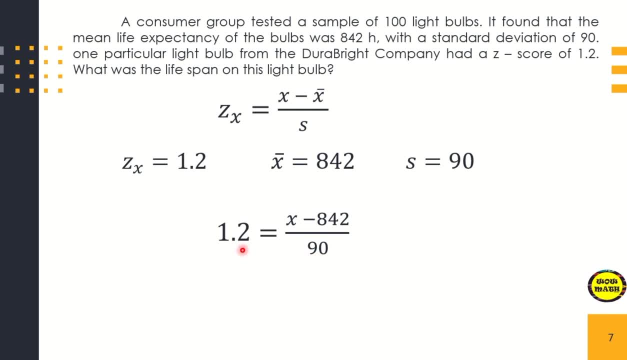 or just simply multiply 90 to 1.2.. So 90 times 1.2,, that is 108,, is equal to x minus 842.. And after that solve for x, So x is equal to 950..